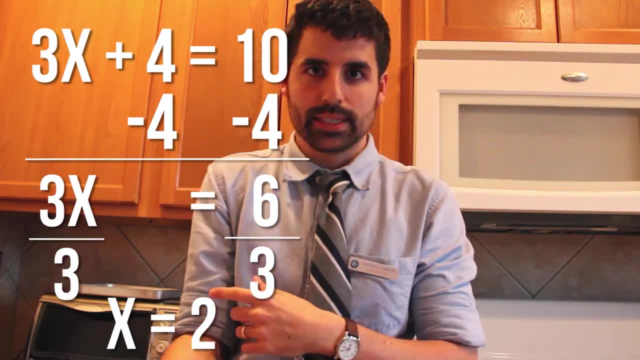 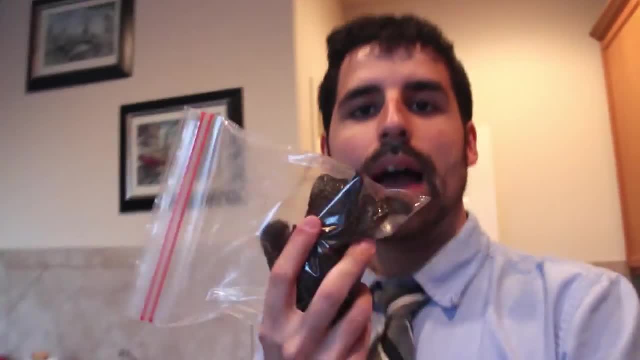 the addition or subtraction first and then take care of the multiplication, because you're just trying to isolate the variable And it worked out okay, but there wasn't like a conceptual understanding of what was going on. I made this beef jerky, by the way, So I found a. 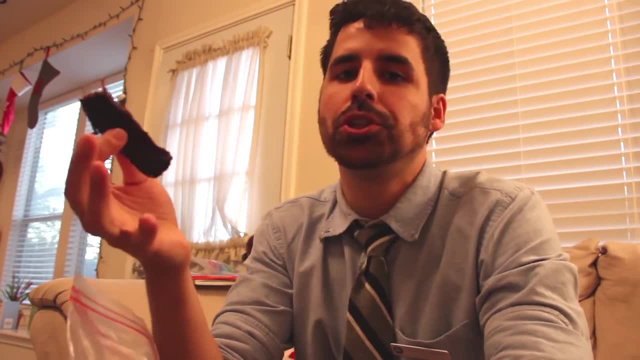 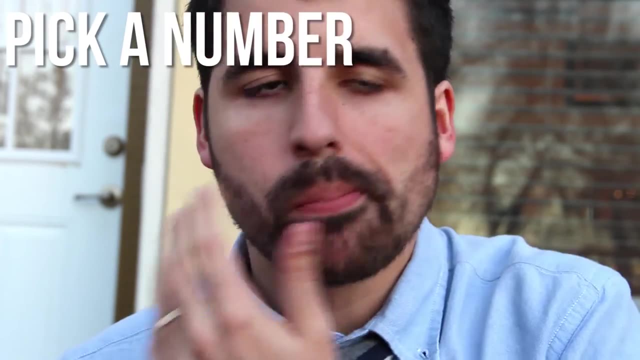 resource that talked about how you can use what they intuitively know how to do in reversing operations to teach the two-step equations. If I tell you to pick a number, multiply it by 2, and then subtract 1, and then say what is your final number, and you said 11.. Students: 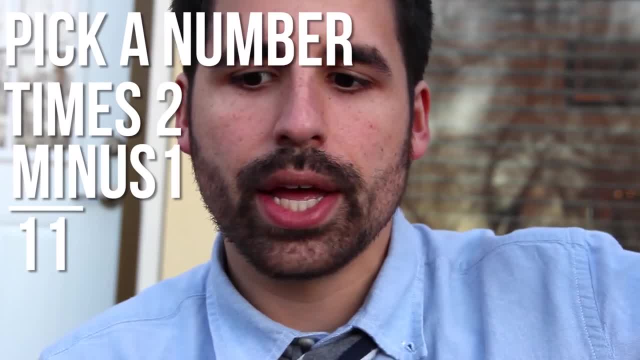 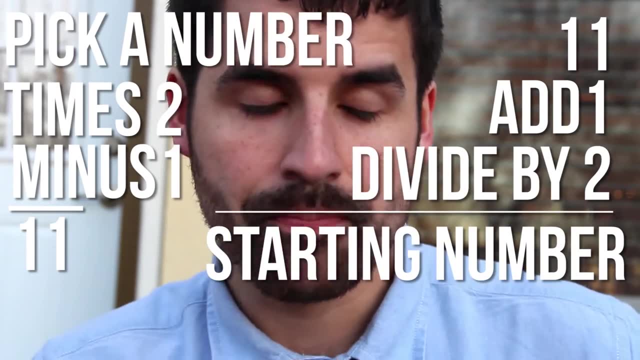 know to intuitively kind of reverse that process, Say, okay, if you multiplied it by 2 and then subtracted 1, that means to get back to where I started. I'm going to have to add 1 and then divide by 2.. I've got to undo what I did. So that's the general premise, And so we're going. 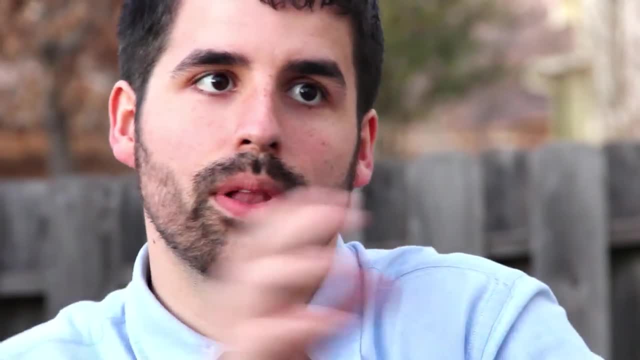 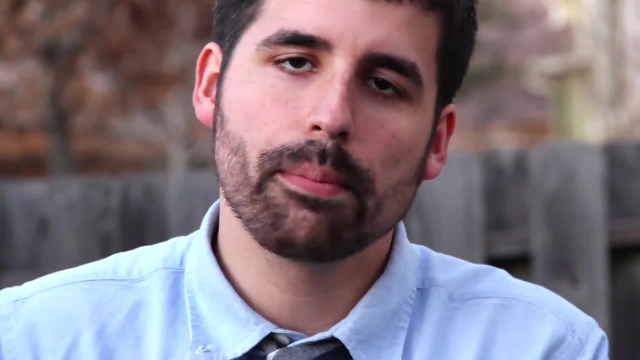 to call it two-step equations. I'm going to start by having them play this math magic game- And I tried it today and it worked fairly well- where I'm just going to have them actually notate the steps and then just whatever mental math they did, Then I plan on taking that process and having them 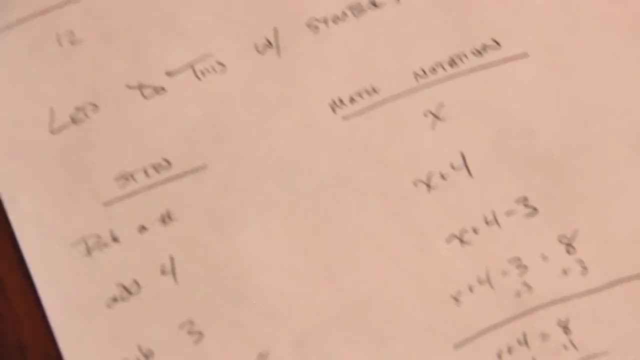 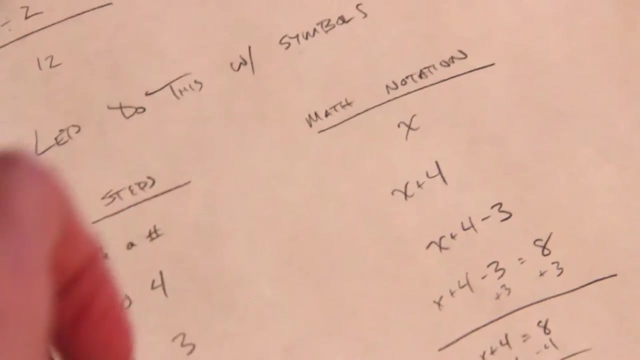 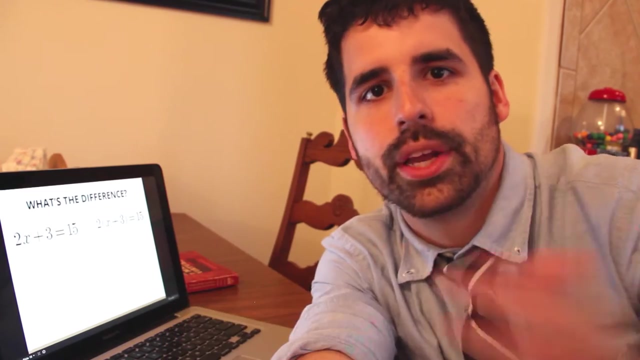 show what it would look like in mathematical notation. We'll go from taking each one of these steps and turning it into mathematical notation, So my hope is to be able to get at the idea that the order of operations is still going to play a role in it. You can't just write. 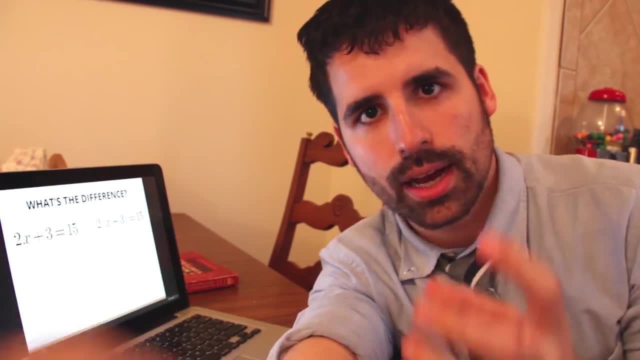 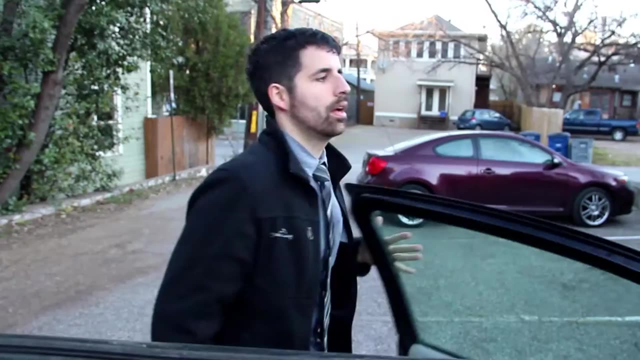 left to right what you're doing and actually realizing. you're taking an unknown number, you're doing something to it and then you're doing something again to it. Let's undo that. We'll see how my other two pre-algebra classes do today. 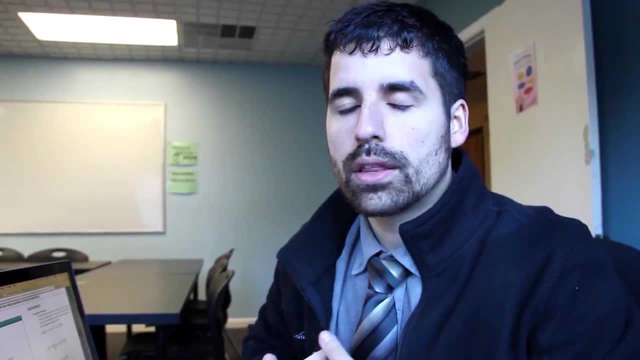 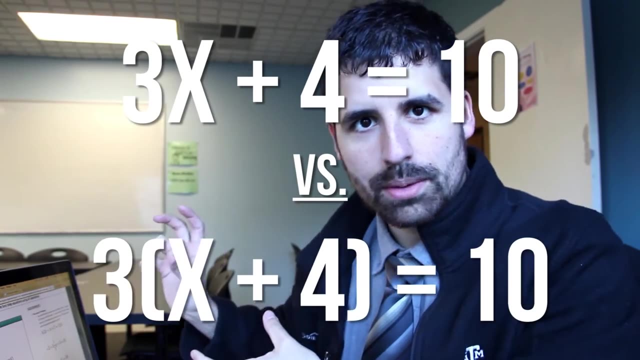 I think the only thing I'll do different is probably have that discussion between when you have the distributive property and when you don't. but it looks like you're using the same terms before I have them kind of practice on their own, making their own. so 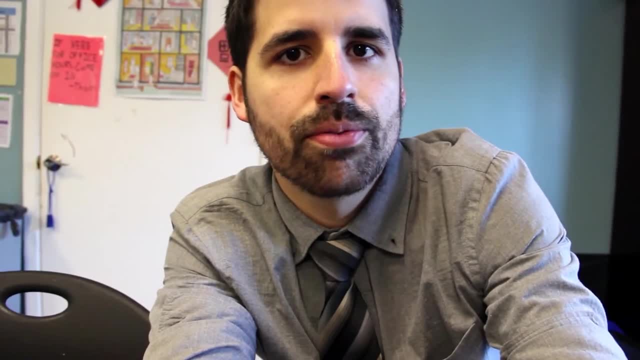 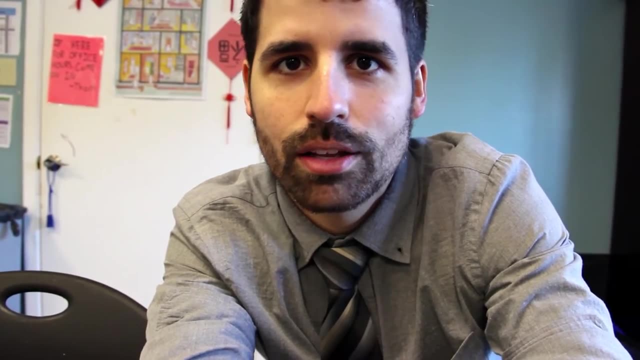 they can see if they're checking it correctly Before we start. there's going to be an auction because my students have a classroom economy. They're all looking at me now. I'll link to the directions and how I do that, But they're. 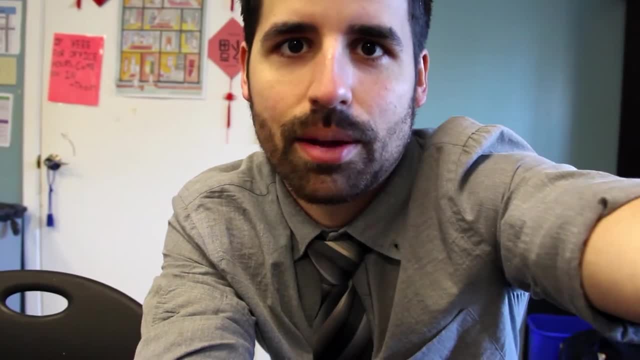 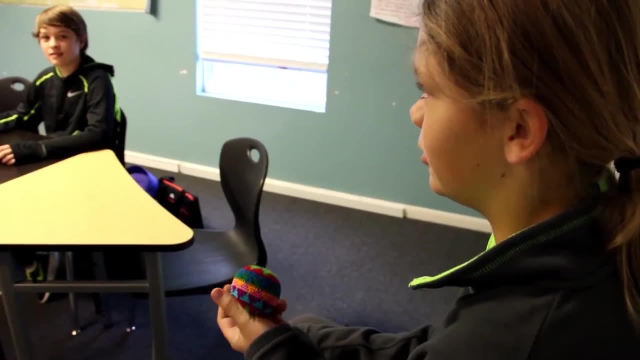 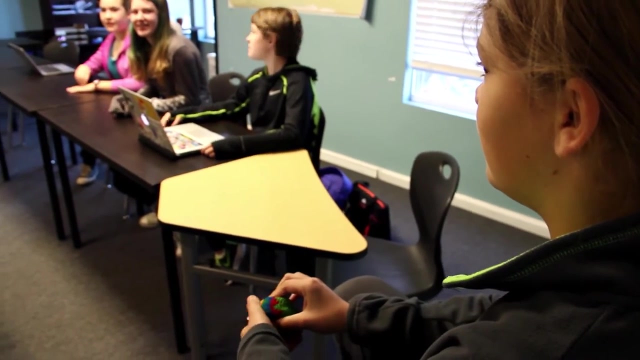 auctioning based on some of the money that they make in the classroom economy. Four items that an auctioneer brought. Remember, you guys do have $500 taxes in April, I know I know Sold to see. you See, I would have gone down at the next hundred. 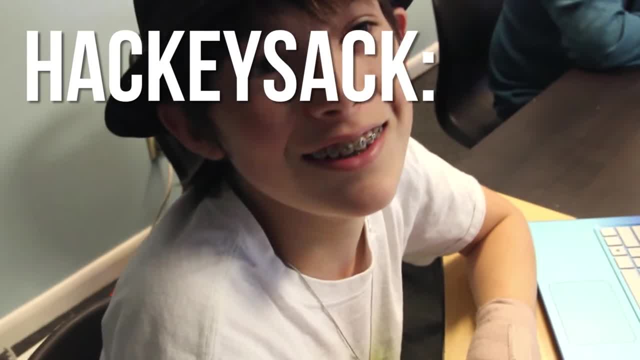 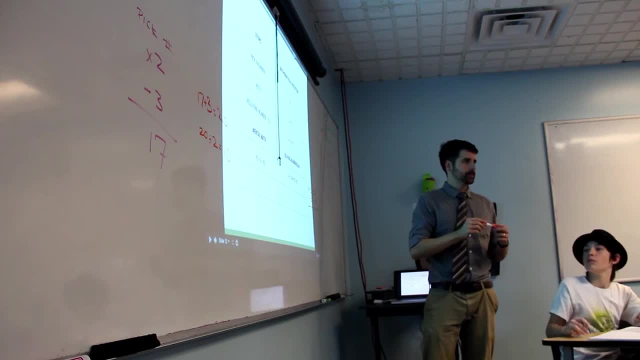 Yeah, how much did you spend on that? At $13,000.. You pick a number and I don't know what you picked. How can I show that mathematically? Nine X, Right, Okay, What? But we don't have to subtract, It's just like. 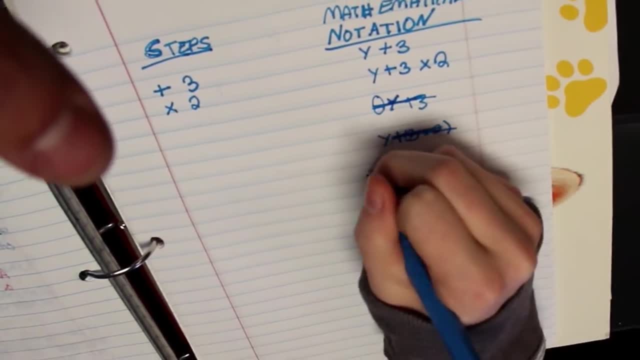 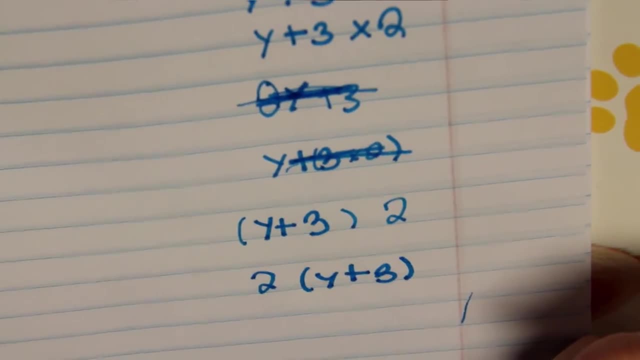 Whenever we want to do something first, okay, write it in the way that we would write it with the distributive property. And if you had said times two plus three, That would have been, That would have. Okay, that makes sense. 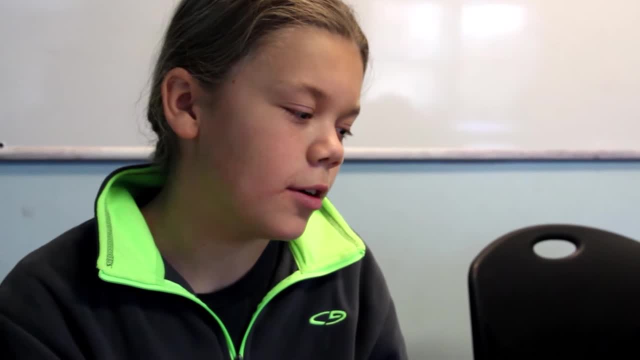 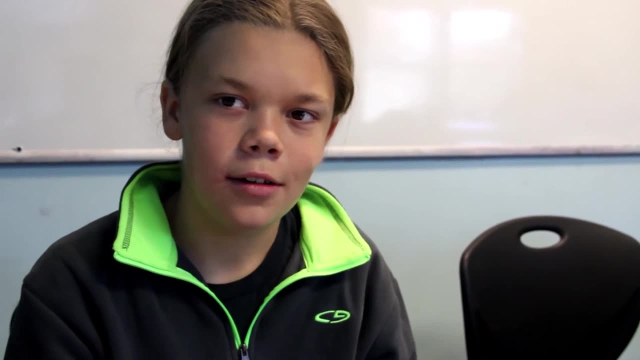 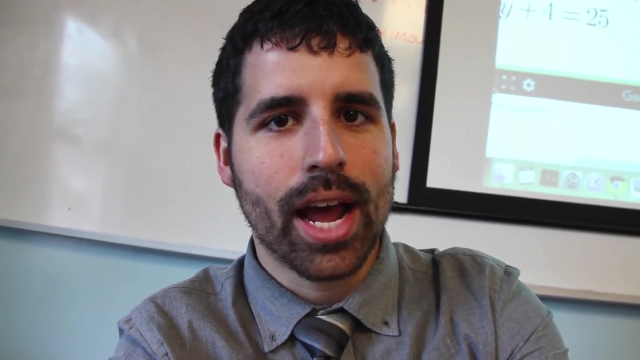 Well, it's like when you have a number and then you multiply it by something. when you're solving algebraically you have to then divide it. It's really hard to show that. It's hard to get them to buy in on actually writing it with mathematical notation Lots. 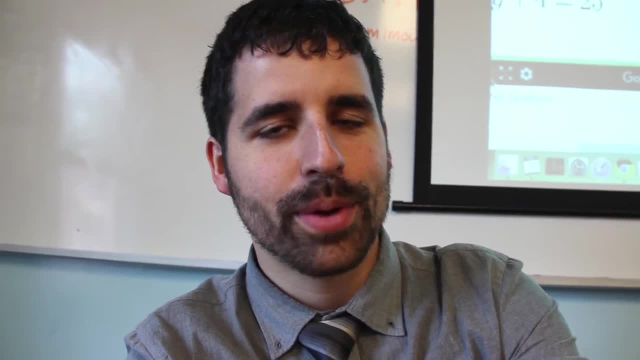 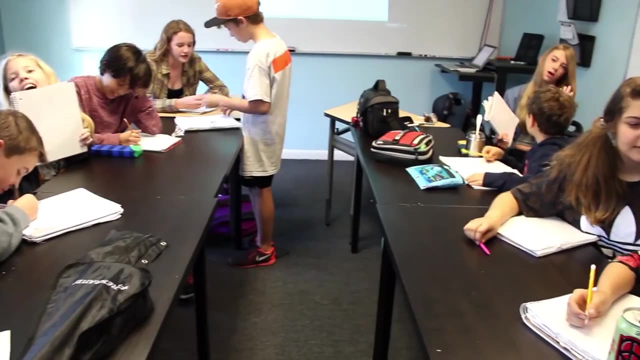 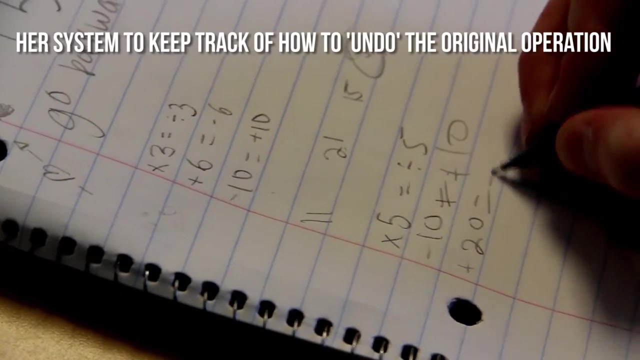 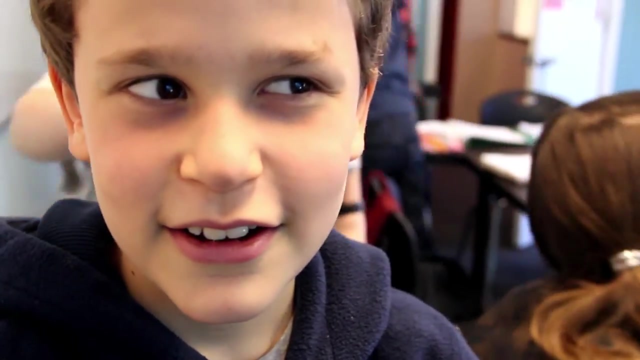 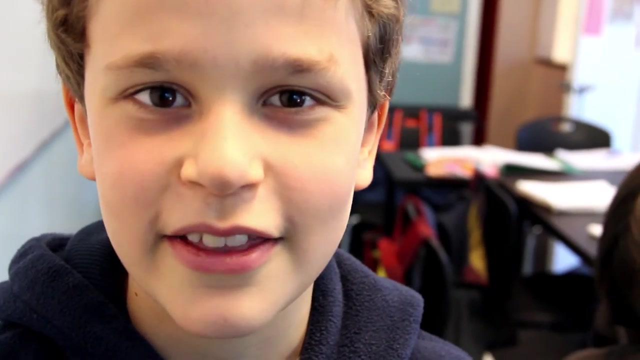 of friction and pushback on writing on mathematical notation, The algebraic way it seems to be, like you know to, It doesn't seem like we need to use it, but as you said, that even though it's hard and it doesn't seem like we need, 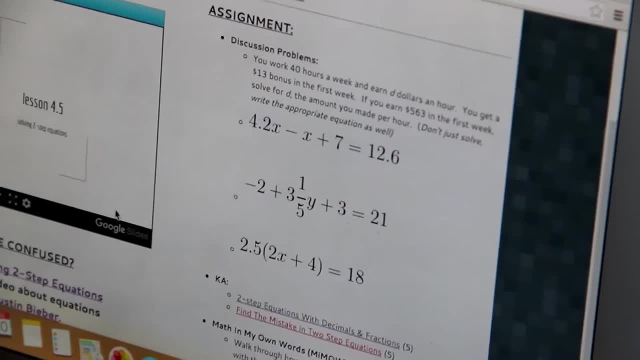 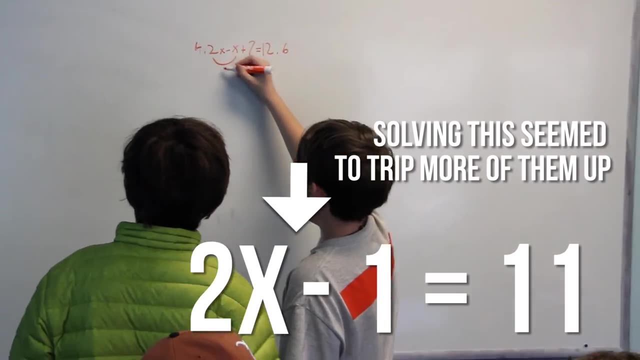 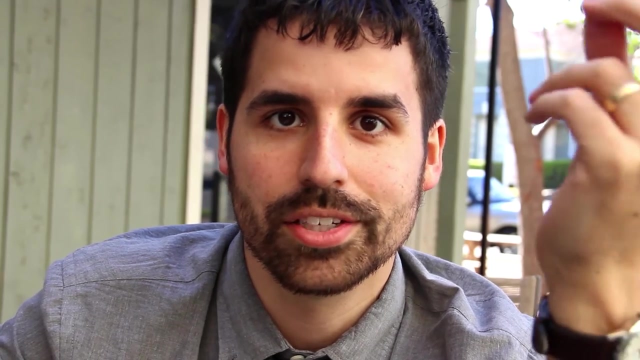 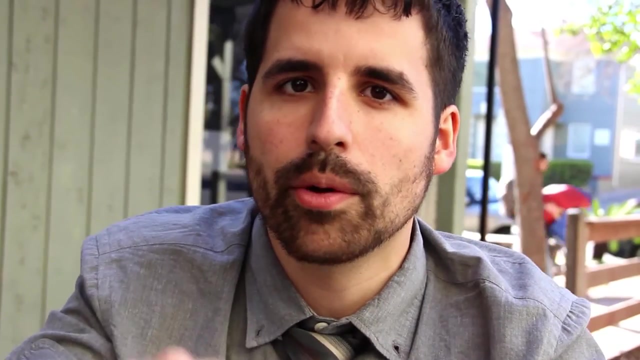 to use it in the future. it'll make things a lot easier for us. So there's definitely resistance to learning how to do mathematical notation. It seems confusing. it's why do it when you don't need to, kind of thing I think they were getting. 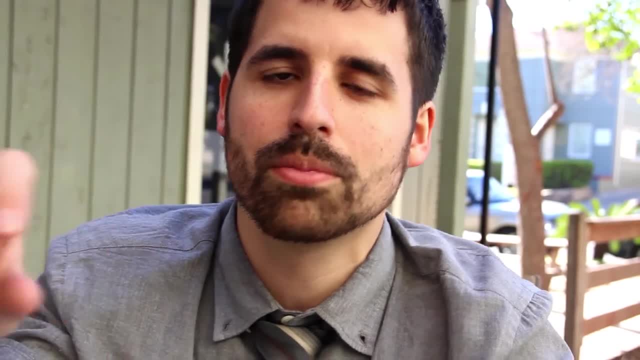 it when we were working with whole numbers. but the thing is like we went straight from working with whole numbers and then I gave them their practice problems, which was working with decimals and fractions and everything, and a lot of them were like God. now I can't. 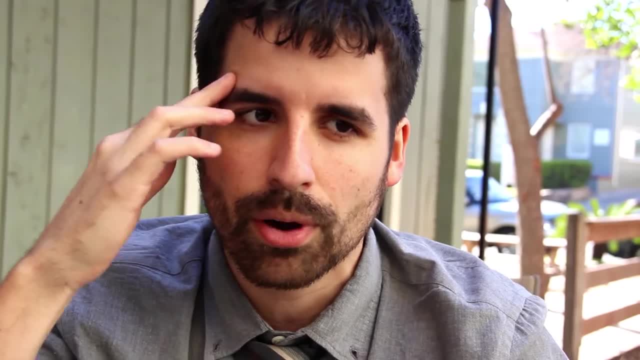 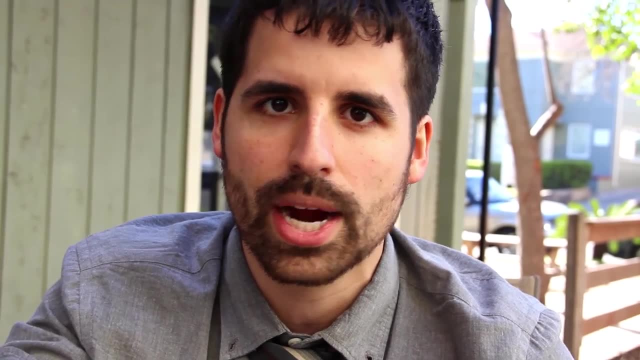 do this in my head and it's really confusing. So I think I would probably scaffold that a little bit, maybe do a couple practice ones together with the decimals, but we'll see how this continues to play out. I think just more practice is going to make them feel a. 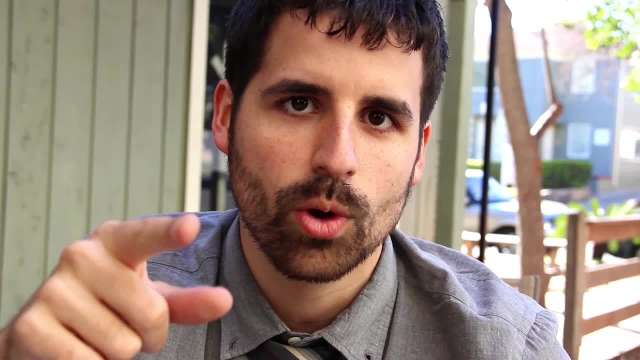 lot more comfortable with it. so they can see what's going on. Thanks for watching. 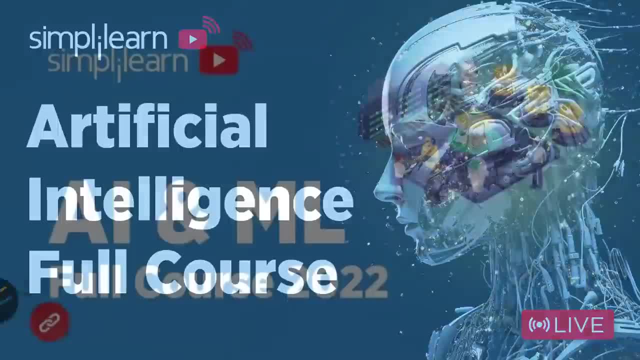 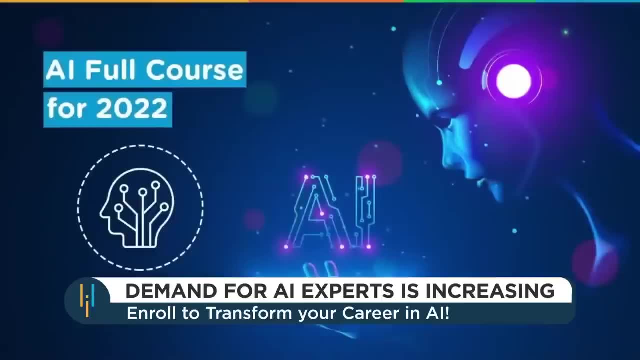 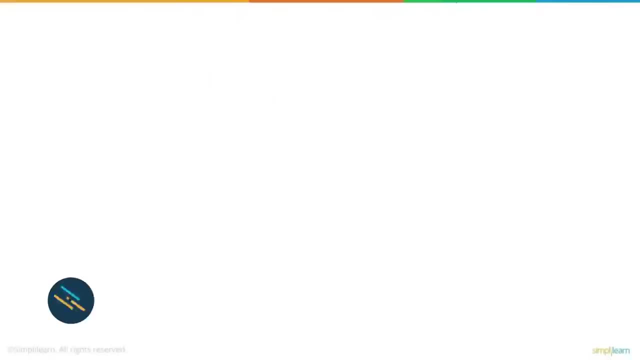 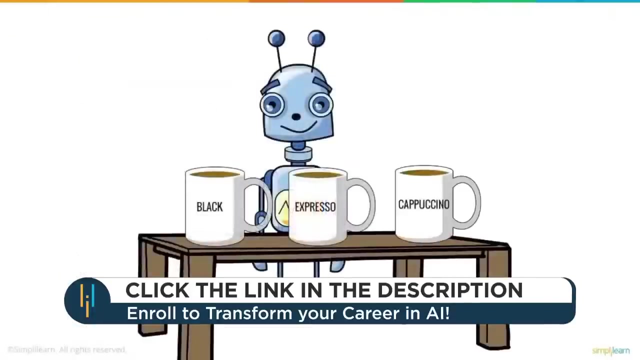 Hi everyone, welcome to this Artificial Intelligence 2022 full course video by SimpliLoan. Artificial Intelligence 2022 full course video by SimpliLoan is an educational video. Please add punctuation in the appropriate places. Hi everyone, welcome to this Artificial Intelligence 2022 full course video by SimpliLoan. 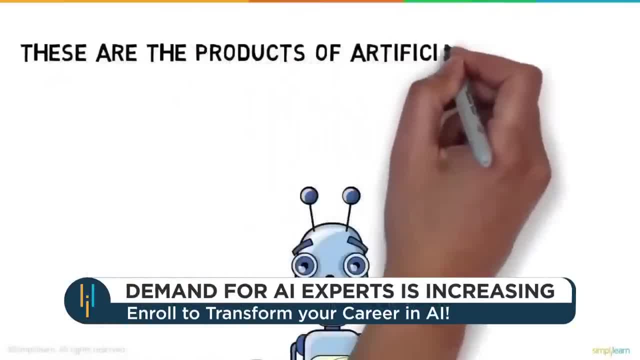 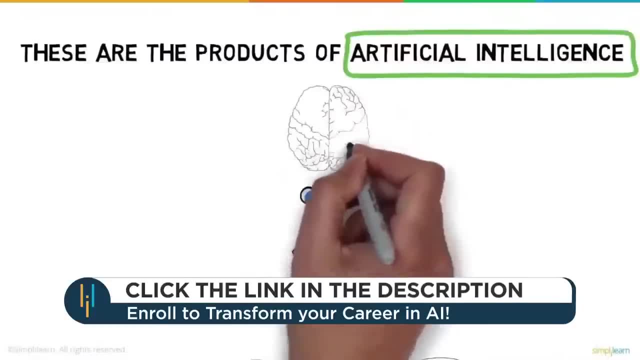 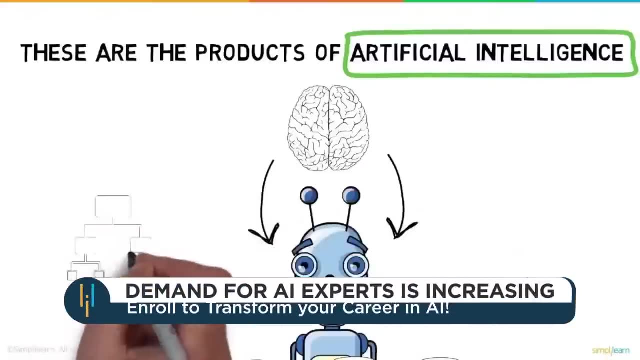 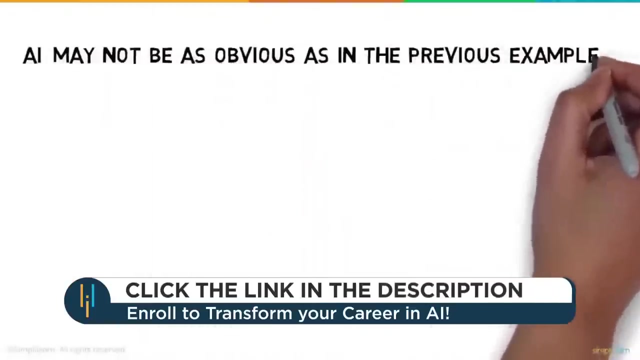